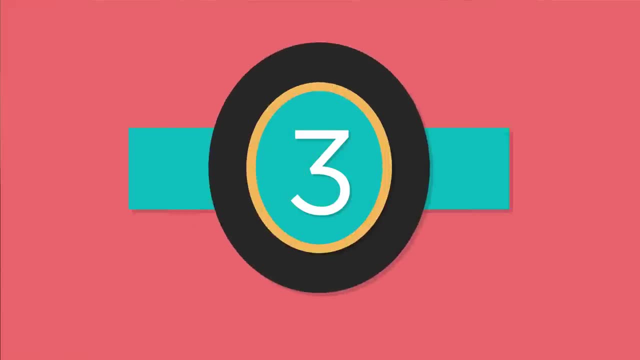 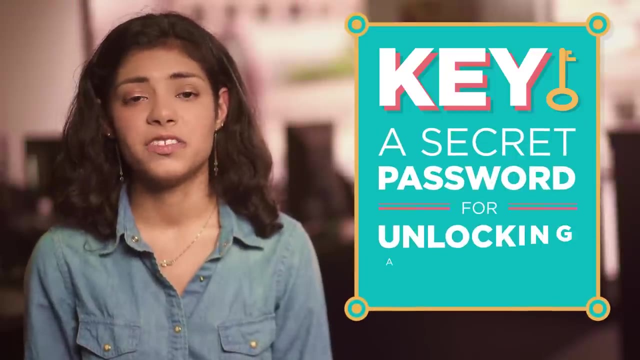 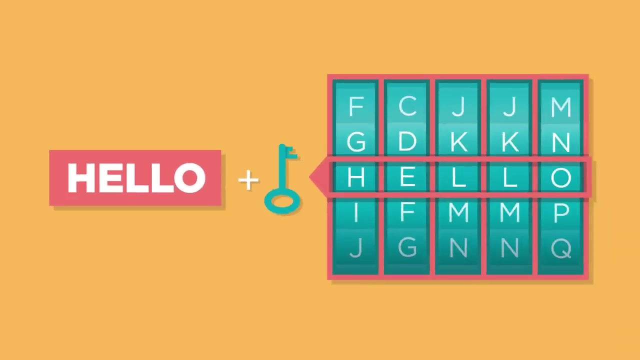 letter a certain number of steps down the alphabet. If the number is something only the sender and receiver know, then it's called the key. It allows the reader to unlock the secret message. For example, if your original message is Hello, then using the Caesar's cipher algorithm with a key of 5, the encrypted message would. 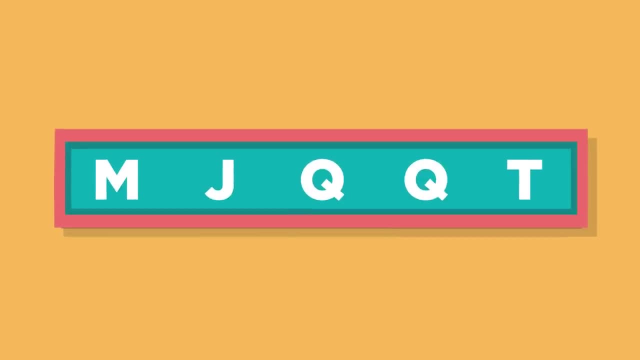 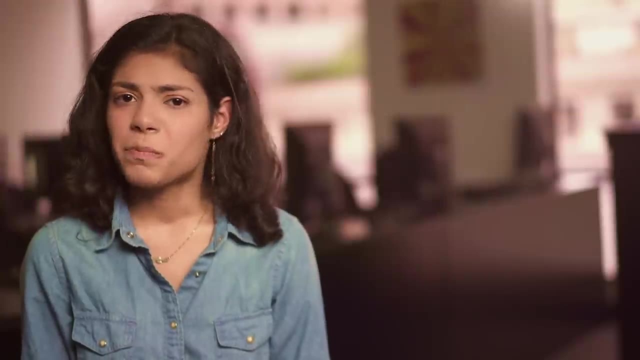 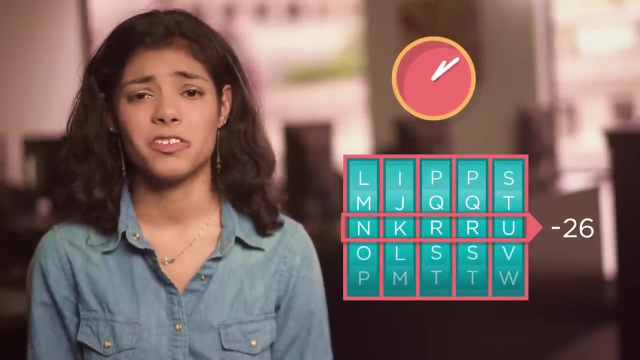 be this: To decrypt the message, the recipient would simply use the key to reverse the process. But there's a big problem with Caesar's cipher. Anybody can easily break or crack the encrypted message by trying every possible key. In the English alphabet, there are only 26 letters. 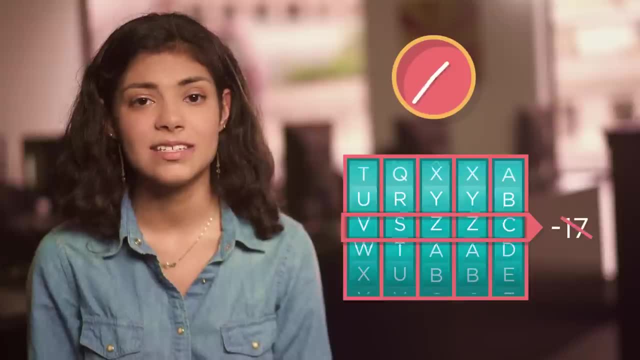 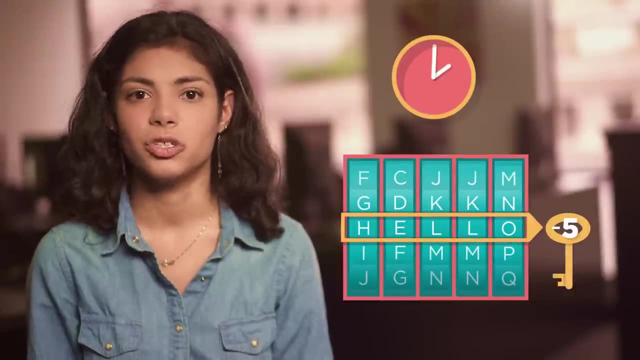 which means you'd only need to try. You'd need at most 26 keys to decrypt the message. Now, trying 26 possible keys isn't very hard. It would take at most an hour to do So. let's make it harder. Instead of shifting every letter by the same amount, let's shift. 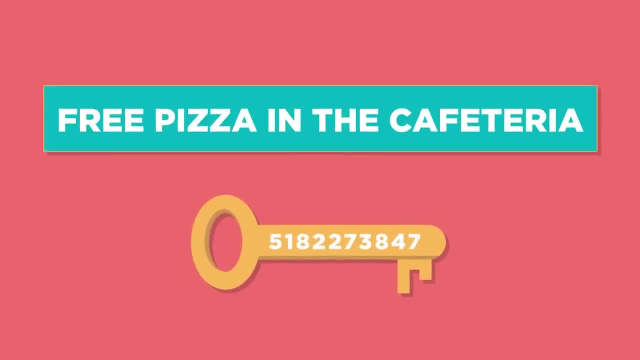 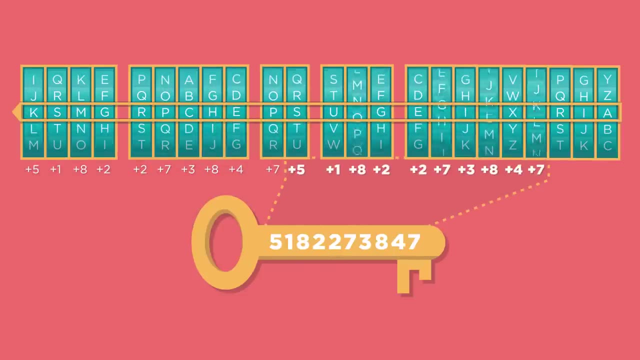 each letter by a different amount. In this example, a 10-digit key shows how many positions each successive letter will be changed to encrypt a longer message. Guessing this key would be really hard. Using 10-digit numbers, you'd need to decrypt the message. But with encryption there could be 10 billion possible key solutions. Obviously that's more than any human could ever solve. It would take many centuries, But an average computer today would take just a few seconds to try all 10 billion possibilities. So in a modern world where the bad guys are armed with computers instead of pencils, how? 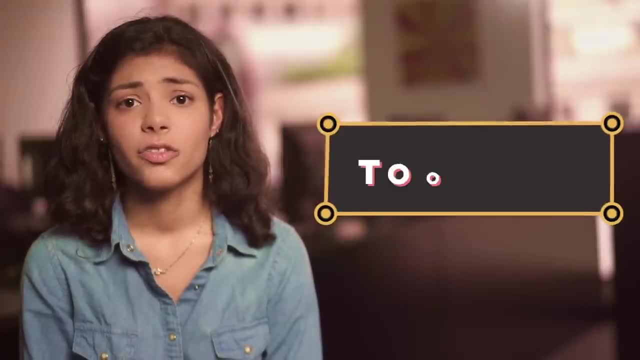 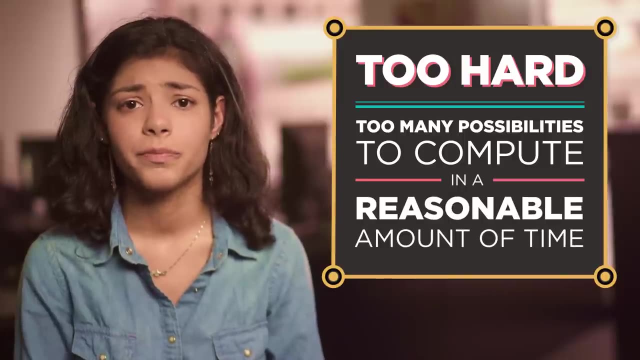 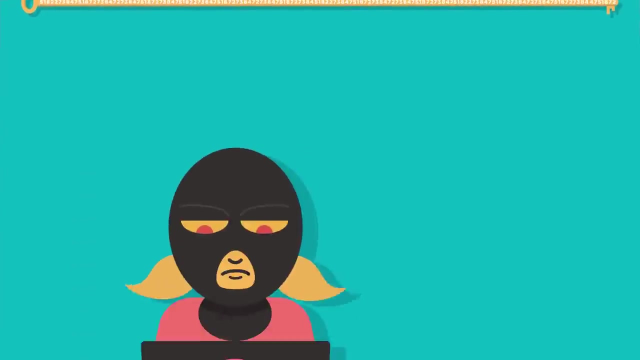 can you encrypt messages so securely that they're too hard to crack? Now, too hard means that there are too many possibilities. The answer is still not clear. Today's secure communications are encrypted using 256-bit keys. That means a bad guy's computer that intercepts your message would need to try this many possible. 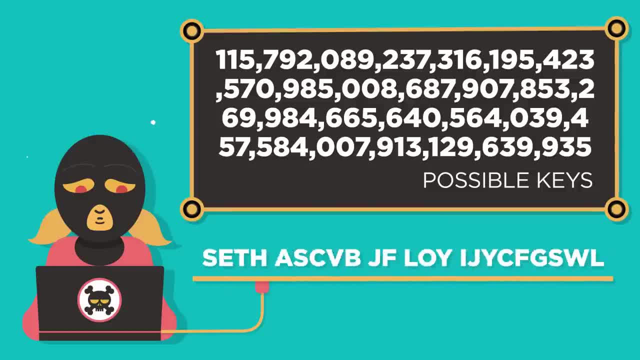 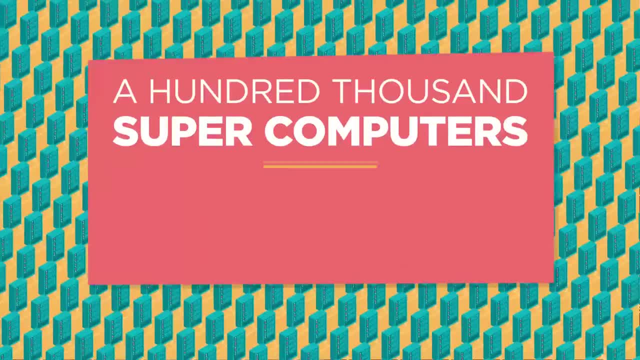 options until they discover the key and crack the message. Even if you had a hundred thousand supercomputers and each of them was able to try a million billion keys every second… It would take at least two years to decrypt a million, two billion, three billion, four. 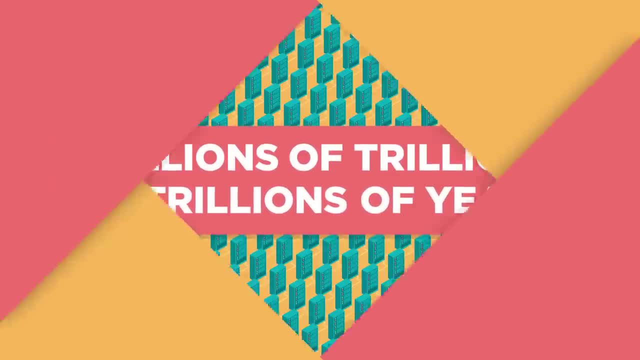 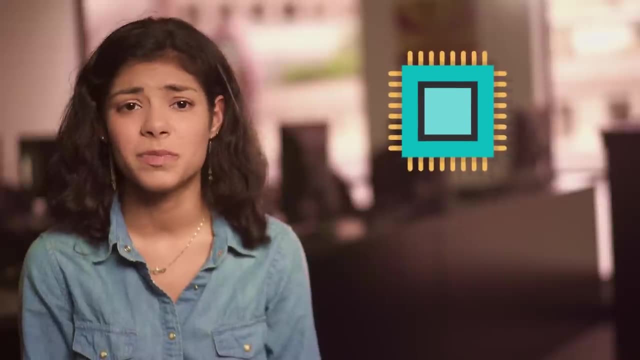 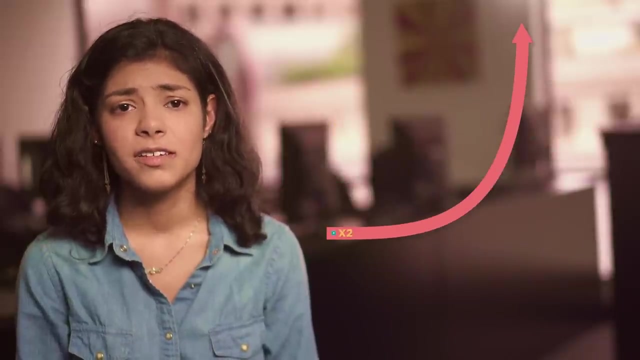 It would take trillions of trillions, of trillions of years to try every option just to crack a single message protected with 256-bit encryption. Of course, computer chips get twice as fast and half the size every year or so. If that pace of exponential progress continues, today's impossible problems will be solvable. 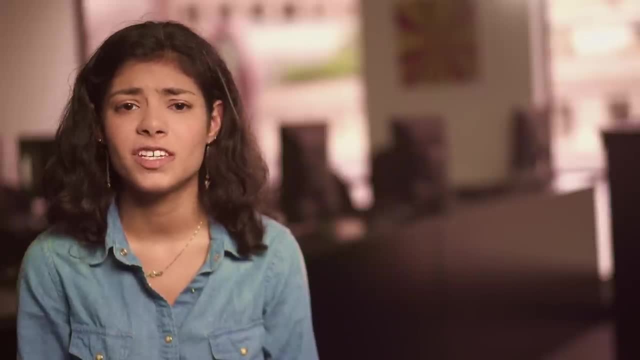 just a few hundred years in the future, and 256 bits won't be enough to be safe. In fact, we've already had to increase the standard key length to keep up with the speed of computers. The good news is, using a longer key doesn't make encrypting messages much harder, but 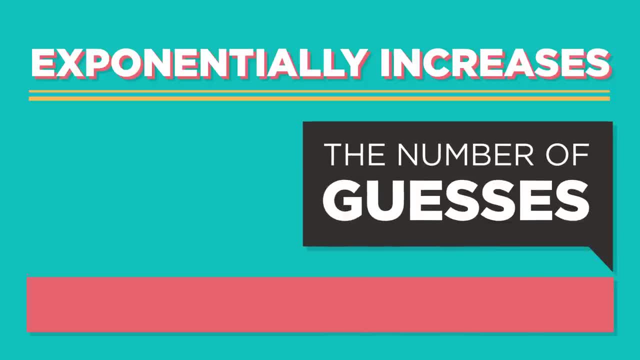 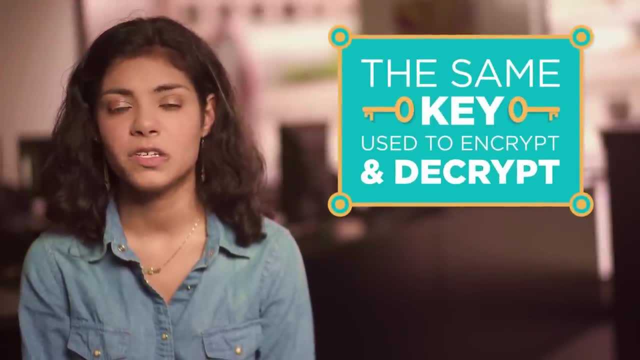 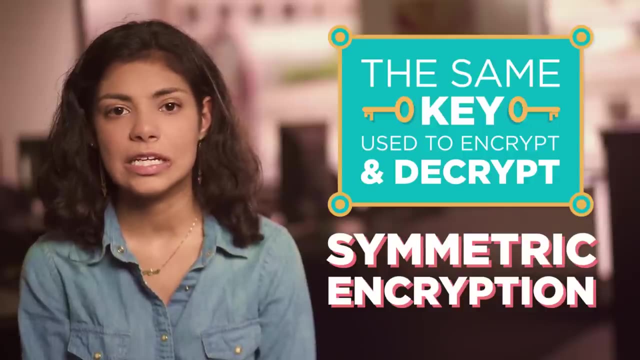 it exponentially increases the number of guesses that it would take to crack a cipher. When the sender and the receiver share the same key to scramble and unscramble a message, it's called symmetric encryption. With symmetric encryption, like Caesar's cipher, the secret key has to be agreed on. 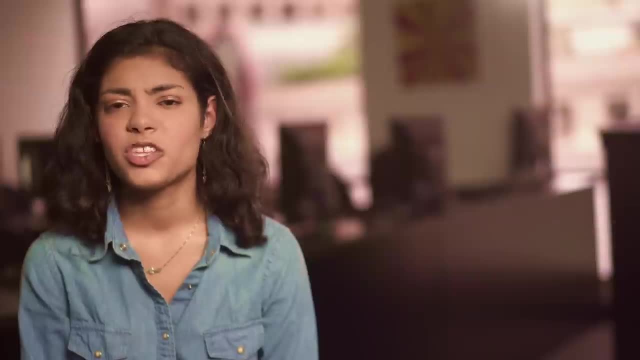 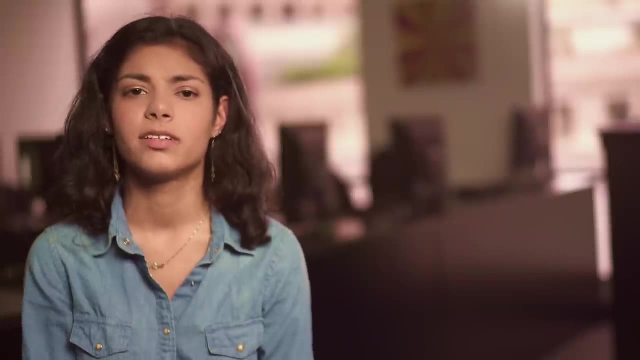 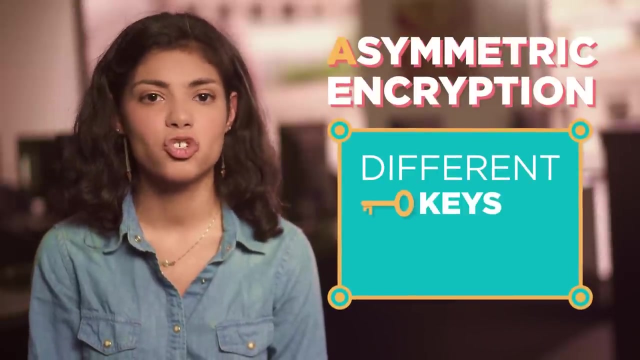 ahead of time by two people in private. That's great for people, but the internet is open and public, so it's impossible for two computers to meet in private to agree on a secret key. Instead, computers use asymmetric keys, a public key that can be exchanged with anybody. 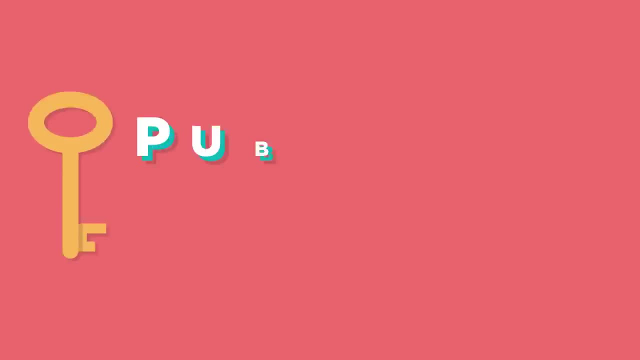 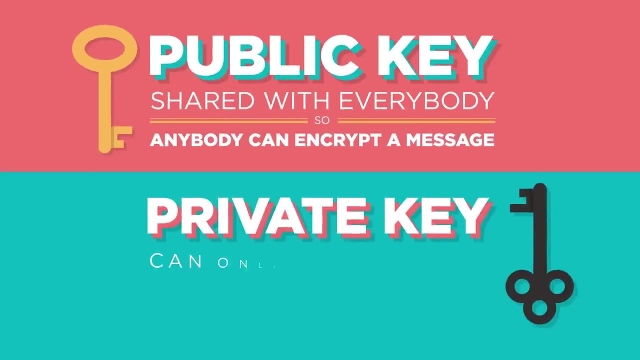 and a private key that is not shared. The public key is used to encrypt data and anybody can use it to create a secret message, But the secret can only be shared with a private key. The secret can only be shared with a private key. 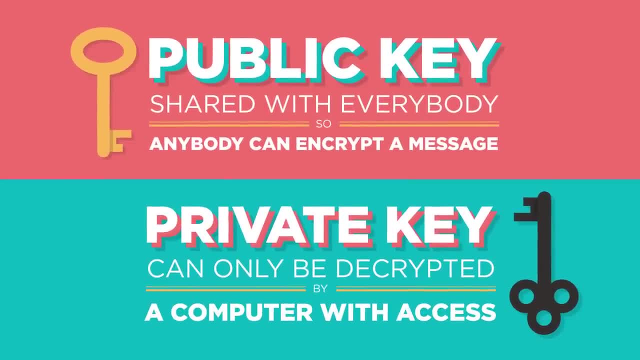 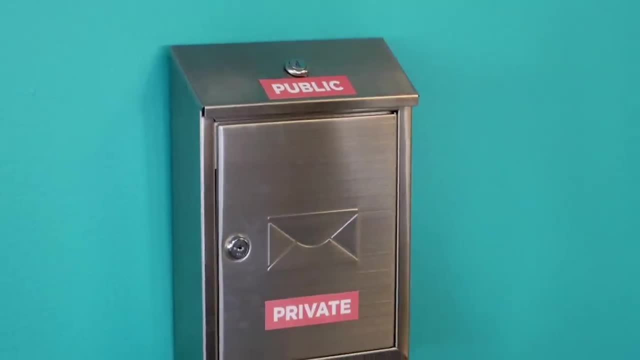 The secret can only be decrypted by a computer with access to the private key. How this works is with some math that we won't get into right now. Think of it this way: Imagine that you have a personal mailbox where anybody can deposit mail, but they need a. 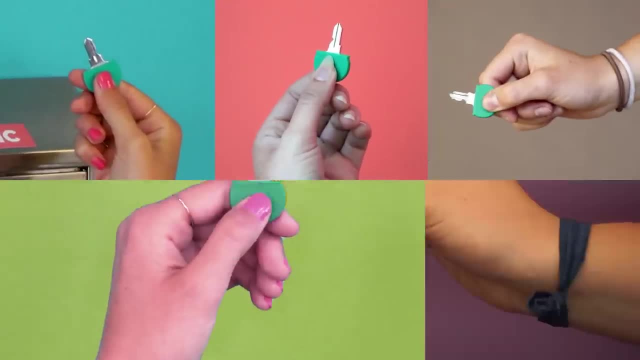 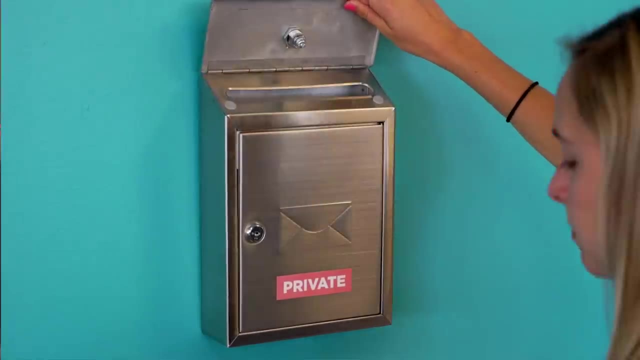 key to do it. You could make many copies of the deposit key and send one to your friend, or even just make it publicly available. Your friend or even a stranger can use the public key to access your deposit slot and drop a message in. 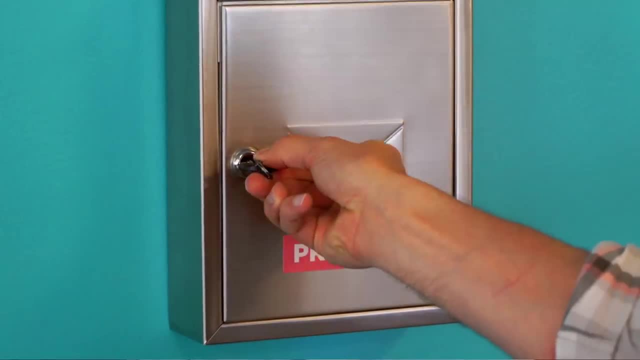 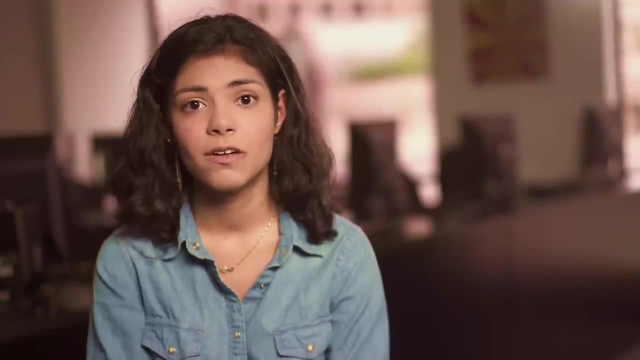 But only you can open the mailbox. You can open the mailbox with your private key to access all of the secret messages you've received, And you can send a secure message back to your friend by using the public deposit key to their mailbox. This way, people can exchange secure messages without ever needing to agree on a private. 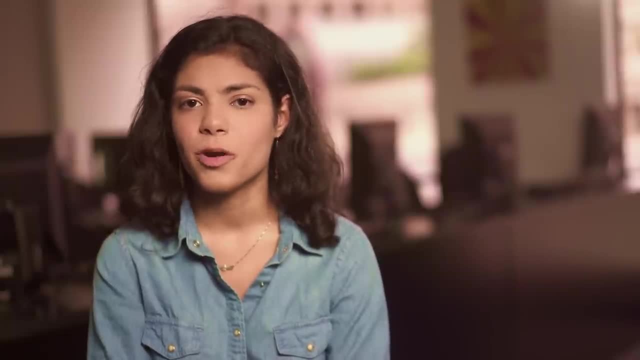 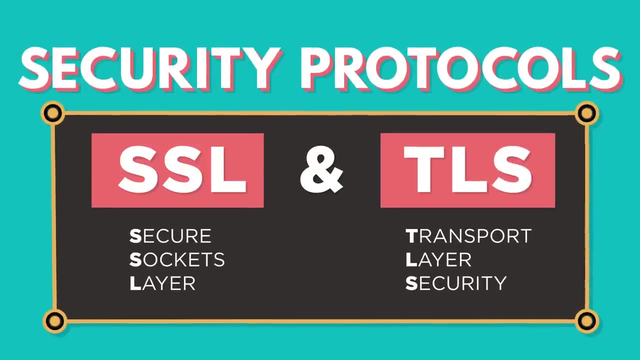 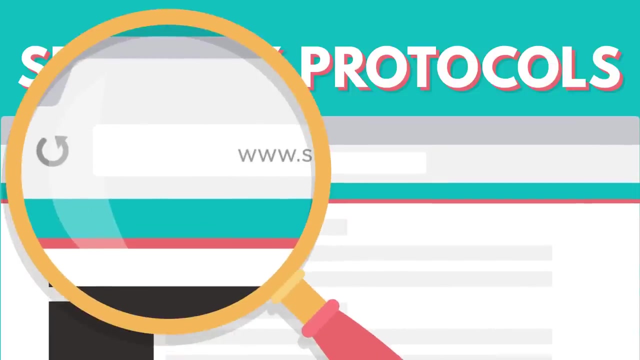 key. Public key cryptography is the foundation of all secure messaging on the open internet, including the security protocols known as SSL and TLS, which protect us when we're browsing the web. Your computer uses this today. anytime you see the little lock or the letters HTTPS in.